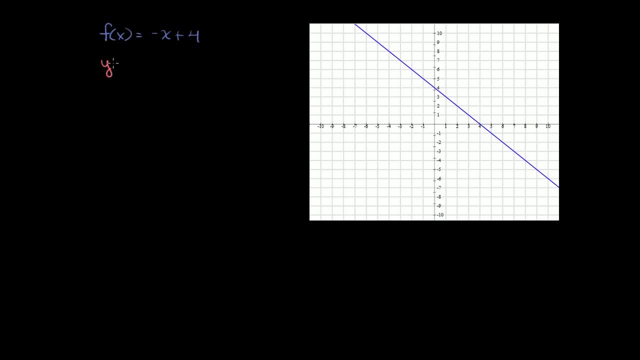 I set the variable y equal to f of x. Or we could write that y is equal to negative x plus 4.. Right now, we've solved for y in terms of x. To solve for the inverse, we do the opposite. 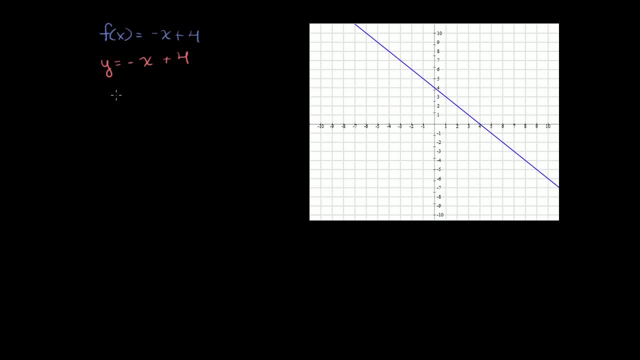 We solve for x in terms of y. So let's subtract 4 from both sides. You get y minus 4 is equal to negative x. And then to solve for x, we can multiply both sides of this equation times negative 1.. 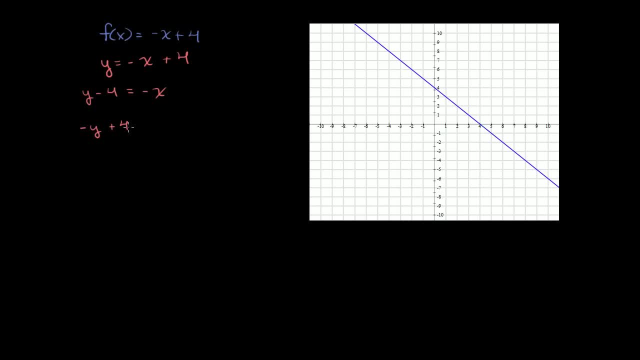 And so you get: negative y plus 4 is equal to x. Or just because we're always used to writing the dependent variable on the left-hand side, we could rewrite this as x is equal to negative y plus 4.. Or another way to write it is: we could. 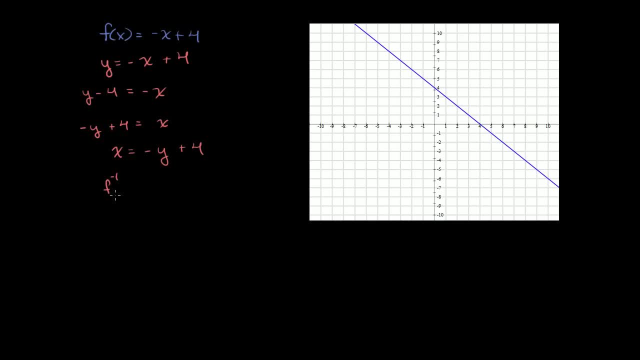 say that f inverse f of x is equal to negative y plus 4.. f inverse of y is equal to negative y plus 4.. So this is the inverse function, right here, And we've written it as a function of y. But we can just rename the y as x. 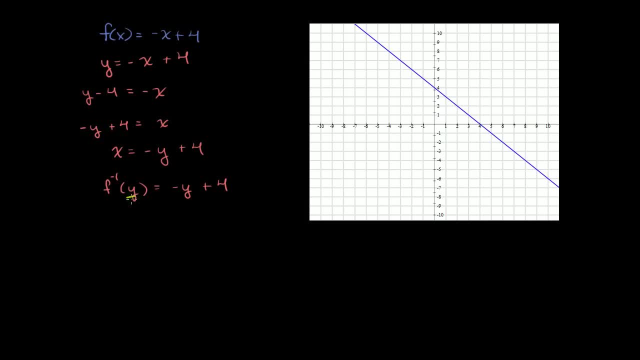 So it's a function of x, So let's do that. So if we just rename this y as x, we get f. inverse of x is equal to negative x plus 4.. These two functions are identical Here. we just use y as the inverse. 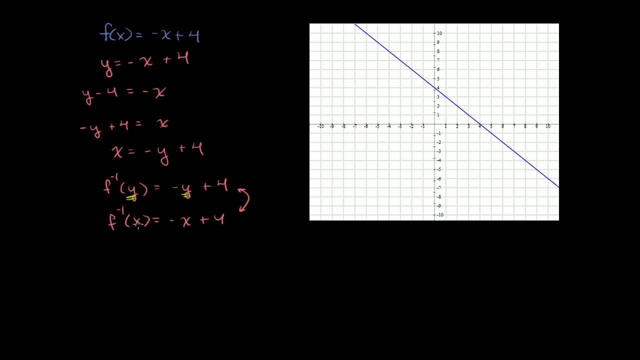 This is the independent variable or is the input variable? Here we just use x, but they're identical functions. Now, just out of interest, let's graph the inverse function and see how it might relate to this one right over here. So if you look at it, it actually 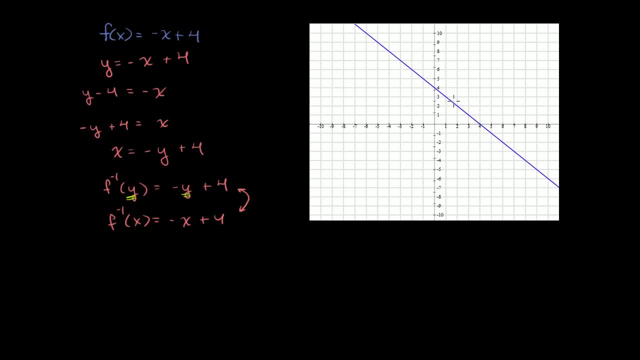 looks fairly identical. It's negative x plus 4.. It's the exact same function. So let's see If we have the y-intercept is 4, it's going to be the exact same thing. The function is its own inverse. 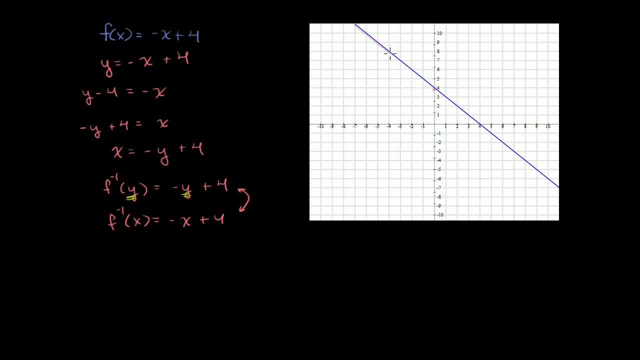 So if we were to graph it, we would put it right on top of this, And so there's a couple of ways to think about it. In the first inverse function video, I talked about how a function and their inverse they are. the reflection over the line y equals x. 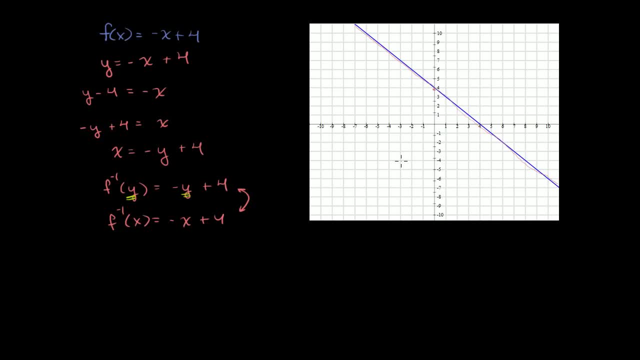 So where is the line y equals x here? Well, the line y equals x looks like this: And negative x plus 4 is actually perpendicular to y, is equal to x. So when you reflect it, you're just kind of flipping it over. 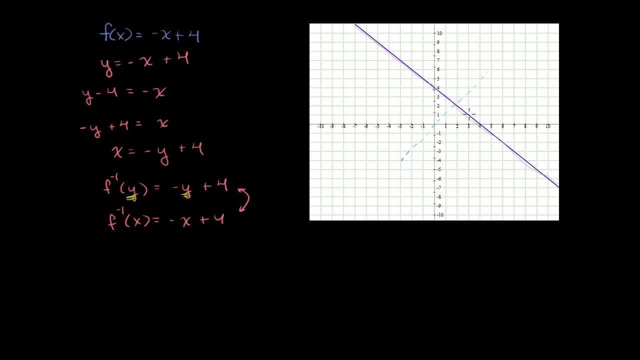 But it's going to be the same line. It is its own reflection And let's make sure that that actually makes sense When we're dealing with, I guess, the standard function right there: if you input a 2, it gets mapped to a 2.. 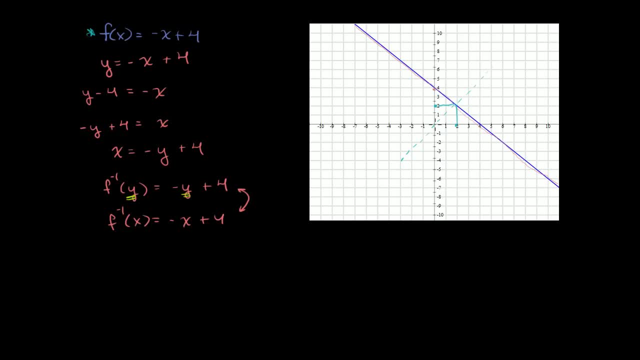 If you input a 4, it gets mapped to 0.. What happens if you go the other way? If you input a 2, well, 2 gets mapped to 2 either way. So that makes sense For the regular function. 4 gets mapped to 0. 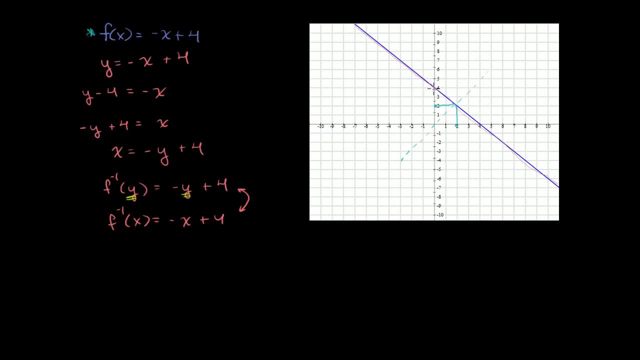 0.. For the inverse function, 0 gets mapped to 4.. So it actually makes complete sense. Let's think about it another way. For the regular function, let me write it explicitly down. This might be obvious to you, but just in case it's not, 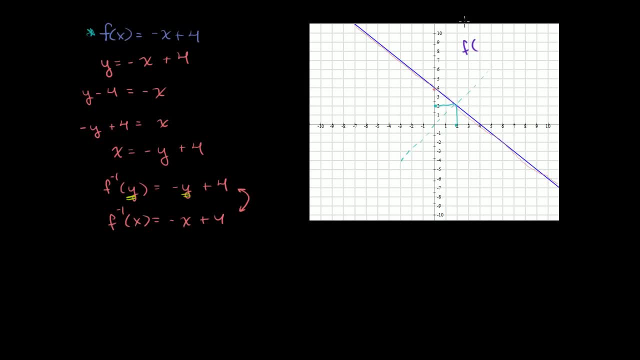 it might be helpful. So let's pick f of 5.. f of 5 is equal to negative 1. Or we could say: the function f maps us from 5 to negative 1.. Now what does f inverse do? What's f inverse? 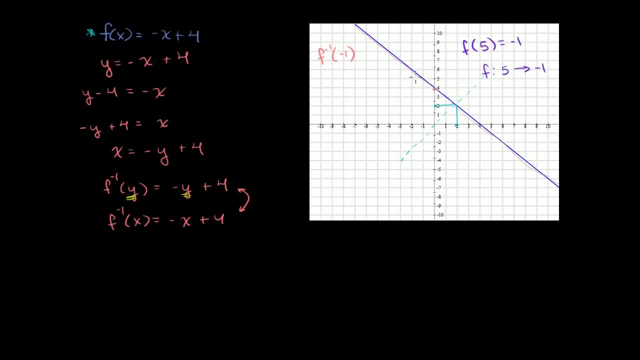 f- inverse of negative 1.. f inverse of negative 1 is 5, is equal to 5.. Or we could say that f maps us from negative 1 to 5.. So, once again, if you think about the sets, there are domains in our ranges. 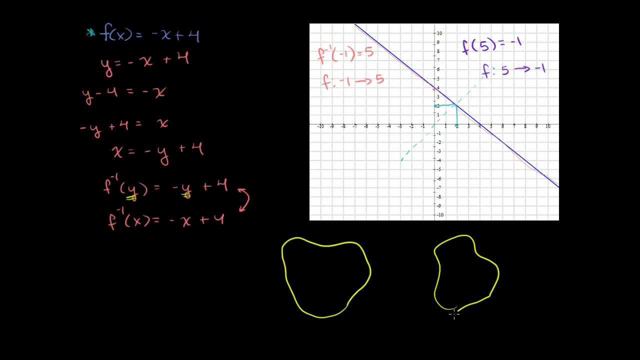 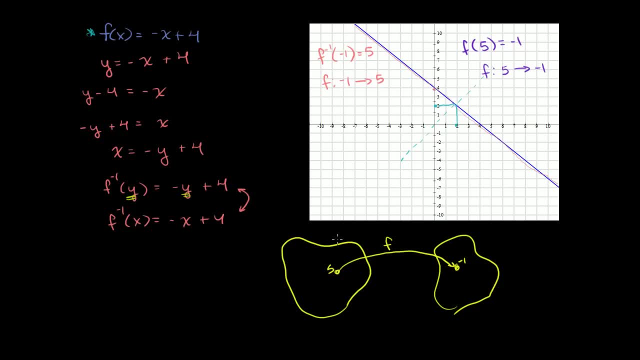 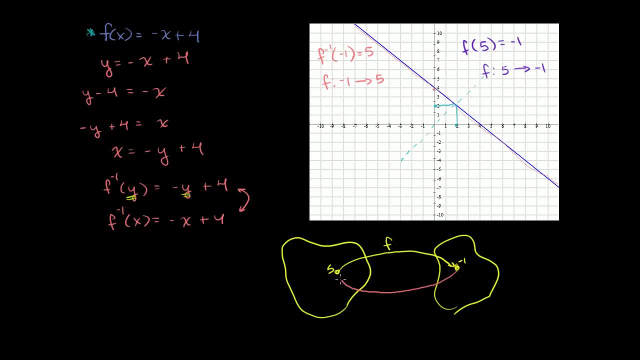 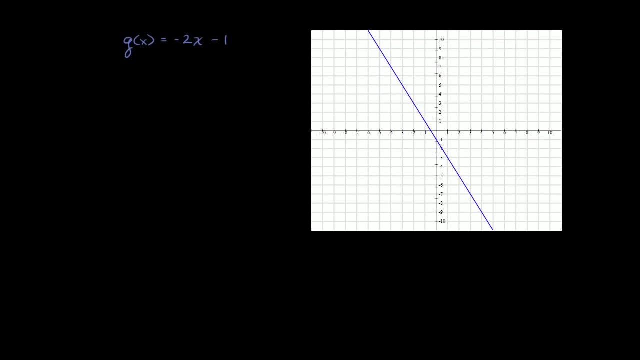 f inverse takes us back from negative 1 to 5, just like it's supposed to do. Let's do one more of these. So here I have: g of x is equal to negative 2x minus 1.. So, just like the last problem, I like to just set y equal to this. 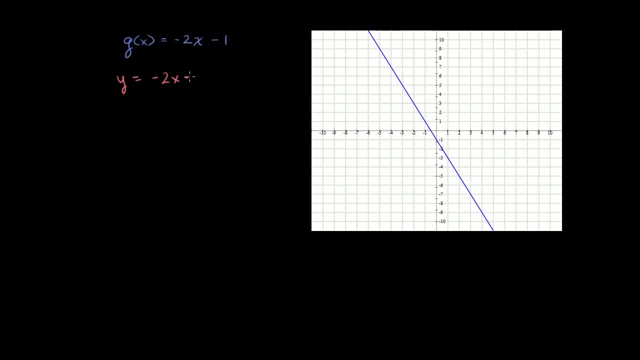 So we say y is equal to g of x, which is equal to negative 2x minus 1.. Now we just solve For x: y plus 1 is equal to negative 2x, Just added 1 to both sides. 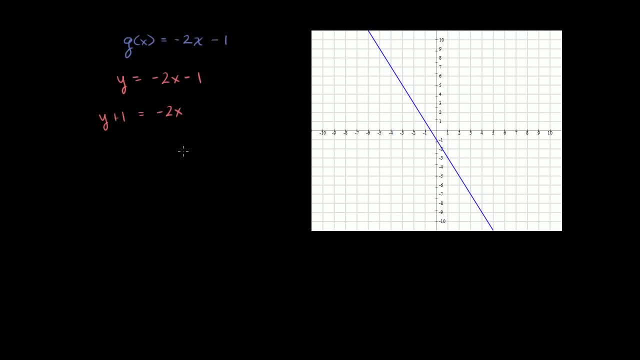 Now we can divide both sides of this equation by negative 2. And so you get negative y over 2 minus 1 half is equal to x. Or we could write: x is equal to negative y over 2 minus 1 half, Or we could write f inverse as a function of y is equal to negative. 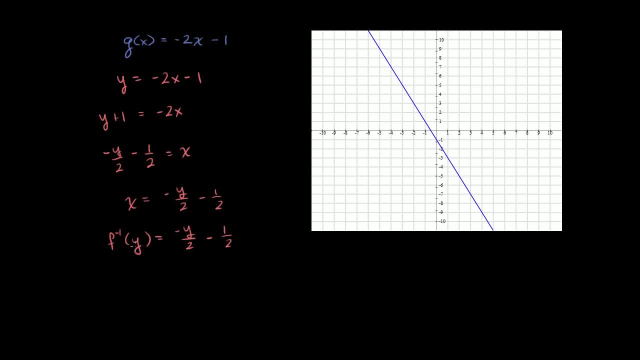 y over 2 minus 1.. x is equal to negative y over 2 minus 1 half. Or we could just rename y as x And we could say that f inverse of- oh, let me be careful here, That shouldn't be an f. 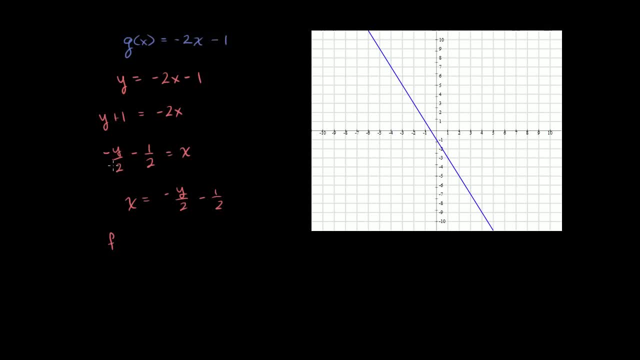 The original function was g. So let me be clear. That is g inverse of y. g inverse of y is equal to negative y over 2 minus 1 half This we started with a g of x, not an f of x. 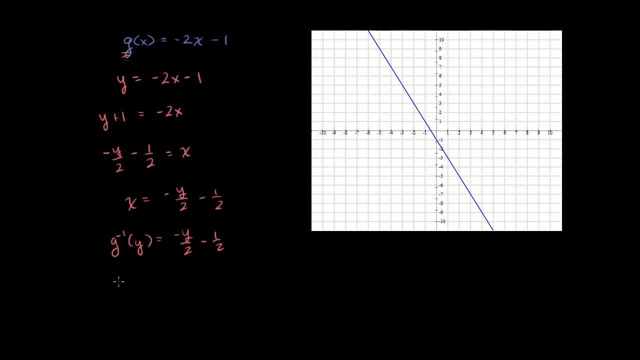 Make sure we get our notation right. Or we could just rename the y and say g minus 1 half. g inverse of x is equal to negative x over 2 minus 1 half. Now let's graph it. It's y-intercept is negative 1 half. so it's right over there. 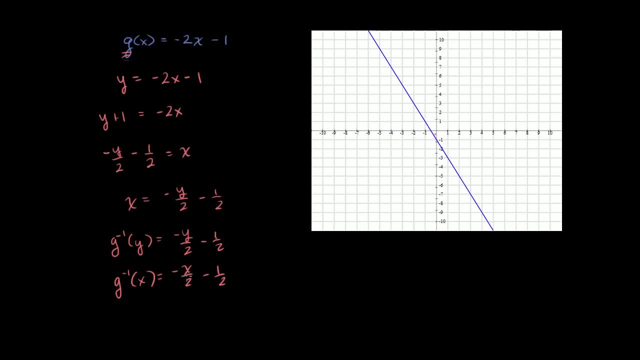 And it has a slope of negative 1 half. It has a slope of negative 1 half. Let's see, if we start at negative 1 half, if we move over to 1 in the positive direction, we'll go down 1 half. 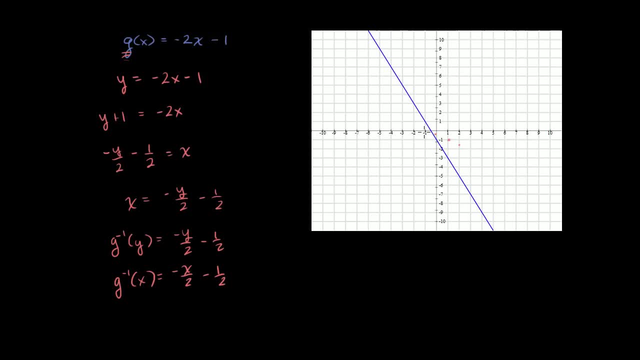 If we move over 1 again, we'll go down 1 half Again if we move back. so we'll go like that. So the line I'll try my best to draw it will look something like that: It'll just keep going.